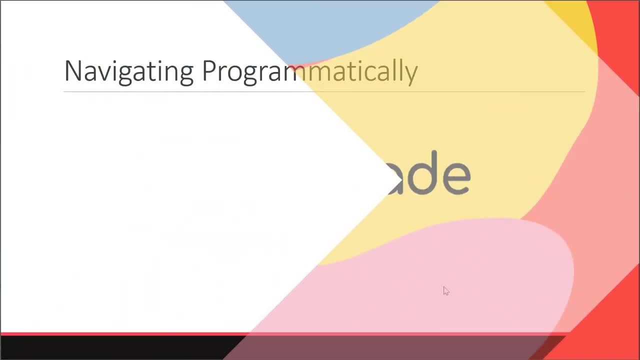 Welcome back. In the previous two videos, we learned how to navigate to different routes using the link and navlink components. For the most part, it is pretty much all you need. However, at times you might need to programmatically navigate to a particular route, For example. 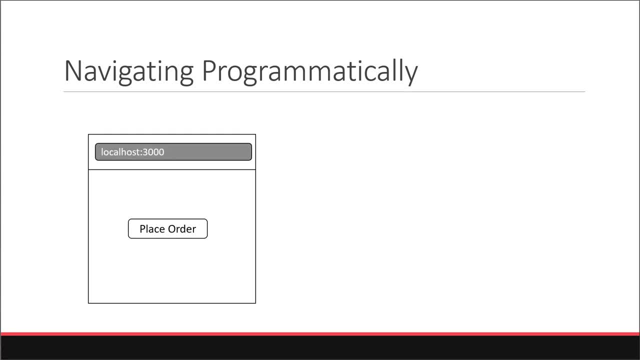 let's say you're placing an order on Amazon. If the form submission is successful, you would be navigated to the order confirmation page. The scenario can hold good for any type of form submission as well and is definitely needed in one or the other application you're. 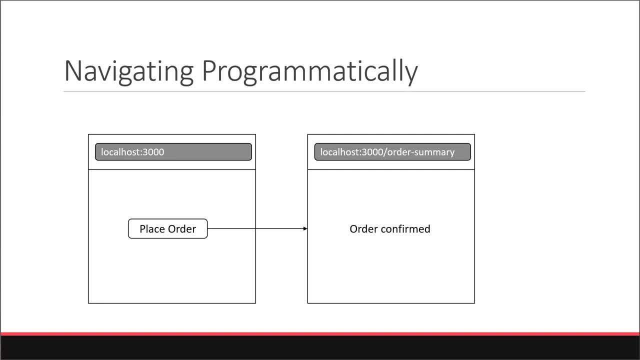 going to build. In this video. let's learn how to do that with React Router. Now we don't have an e-commerce website or a form submission, So let's assume that is the scenario and implement a button click handler where we programmatically navigate to a different route in our application. For our example on click. 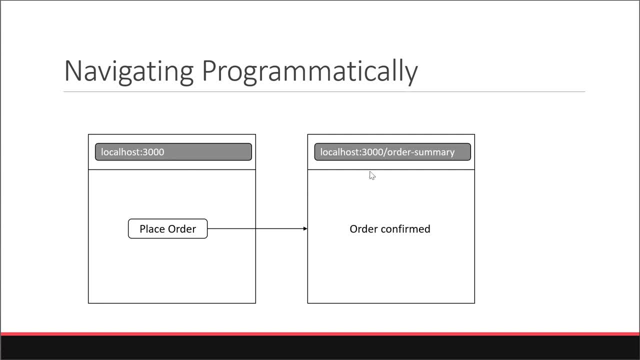 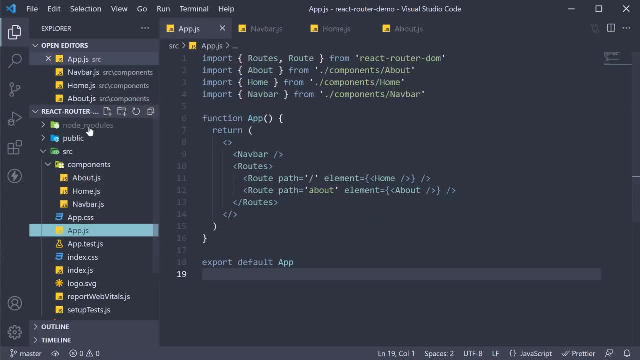 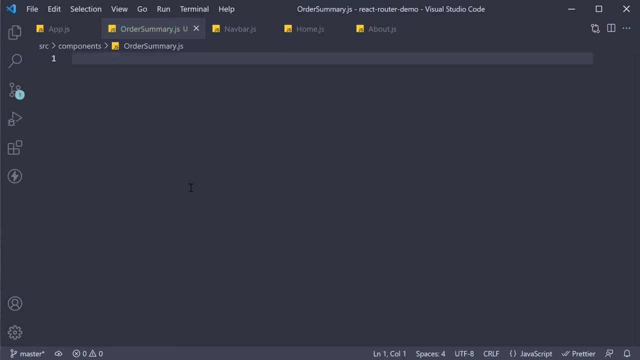 of a place. order button in the home page, let's navigate to the order summary page. Back in VS Code. in the components folder I'm going to create a new file: Summaryjs. Within the file I'm going to create a simple component that reads the: 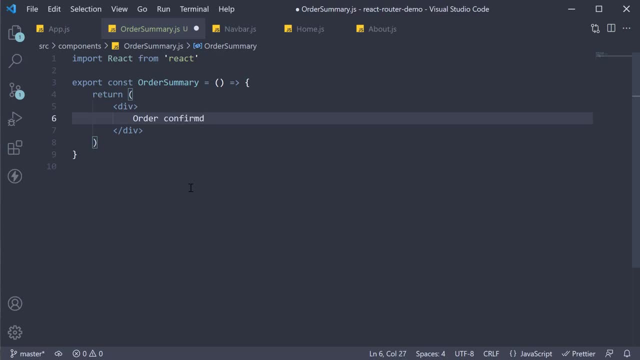 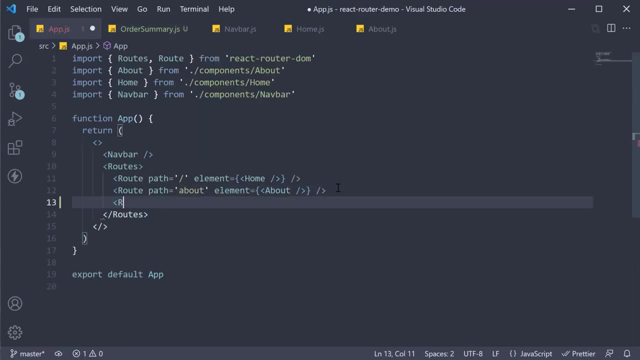 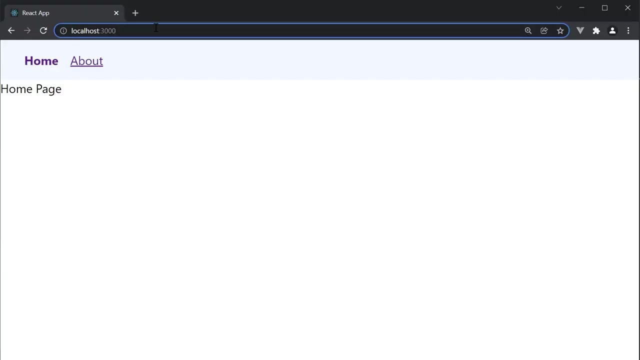 text order confirmed. Next, in appjs I'm going to add a new route. Path is going to be order-summary and the element is going to be equal to the order summary component. Make sure to import the component at the top. If we now head to the browser and navigate to localhost3000 slash order-summary, we should. 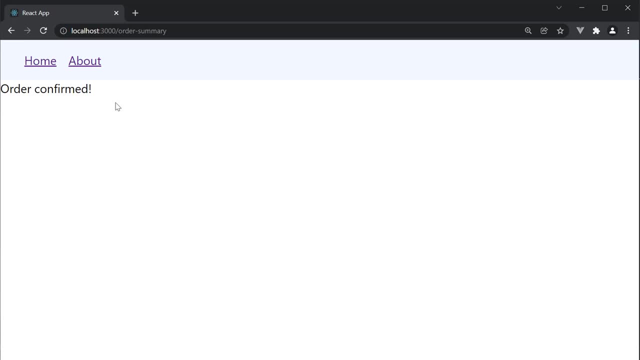 see the text that our order is confirmed. Now, a page like order confirmation isn't something you navigate to on click of a button or a link. It typically happens after an event is successful, For example, placing an order. So let's add a button in the home page that says place. 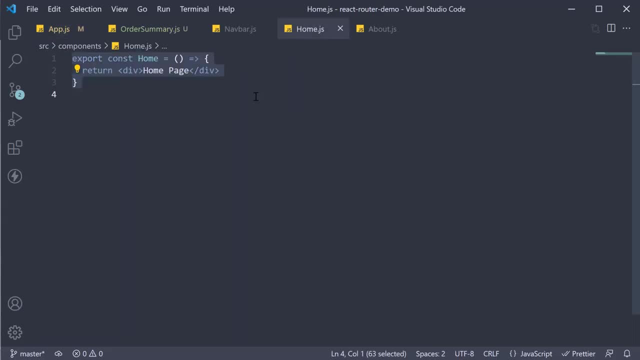 order. So in homejs, wrap the JSX with fragments and add the button Place order. What we want to do is, on click of this button, navigate to the home page and add a button Place order. Now, once you've entered the colleges, you can take a look atstagratasg. just go into. 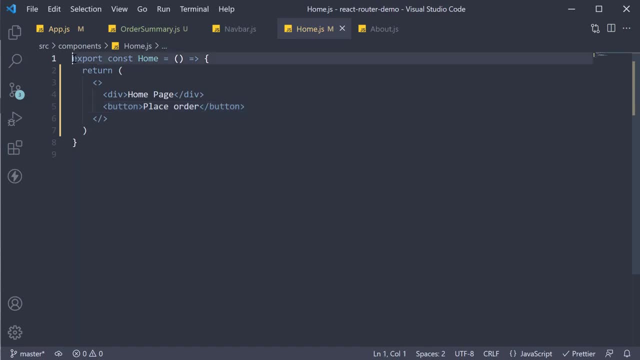 this connection to the order summary page To navigate programmatically: react router provides the USe Navigate hook, So let's import it at the top. Import USeNavigate from react-router-dom and we can now invoke this hook within the component USeNavigate. 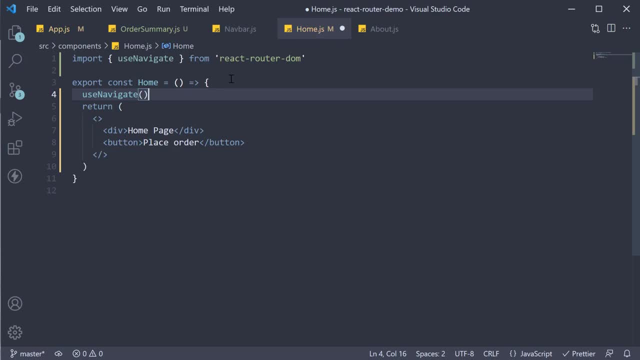 User. I want to turn this off. So if this is not running now, ball hash Doesn't matter, Just wait. So const navigate is equal to use navigate with parentheses. Using this navigate function, we can now navigate to the order summary route on click of the button. So button on click arrow function. 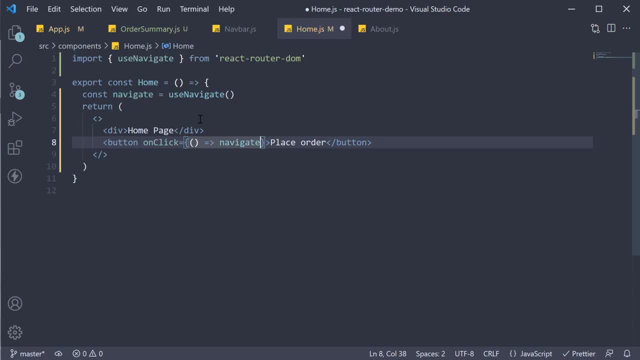 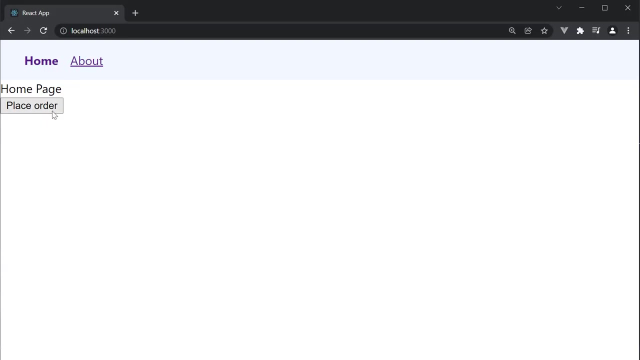 and we call navigate, passing in the path for the route which is order-summary. Let's save the file and test it out. We're in the home page. Click on place order button and we are navigated to the order summary page. The route is order-summary and we see the text order confirmed. We have. 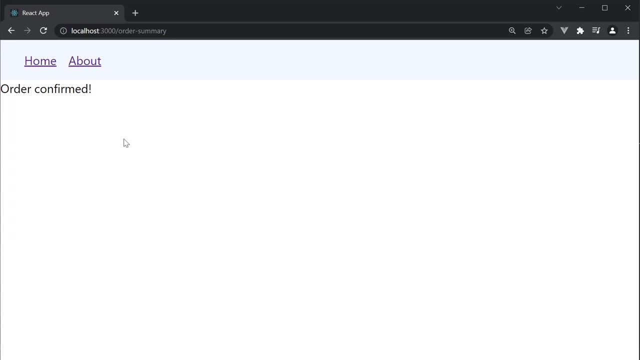 summary: We can now navigate to the route. We can now navigate to the route. We can now navigate successfully, navigated programmatically. Now, implementing a back button programmatically is also done with the use navigate hook. Let me show you how, In order, summary component, I'm going to. 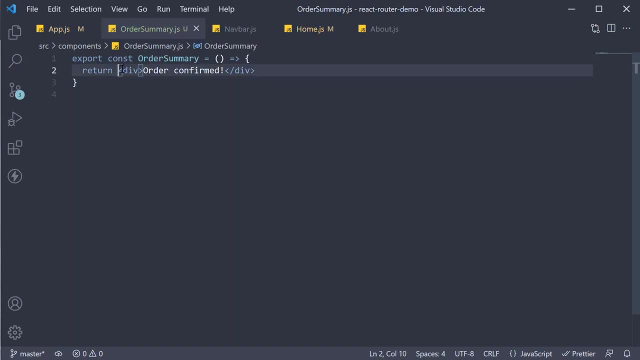 add a back button, So wrap with fragment, and then a button that says go back. Now let's repeat the same steps as before: Import: use navigate hook from react router DOM. Call the hook and assign it to a constant called navigate, which is a function, And on click of the button, call navigate. But this time we simply: 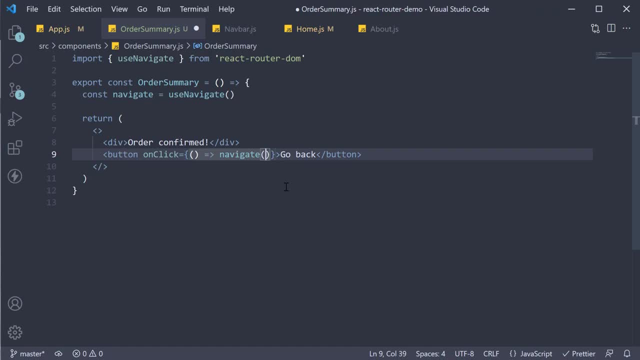 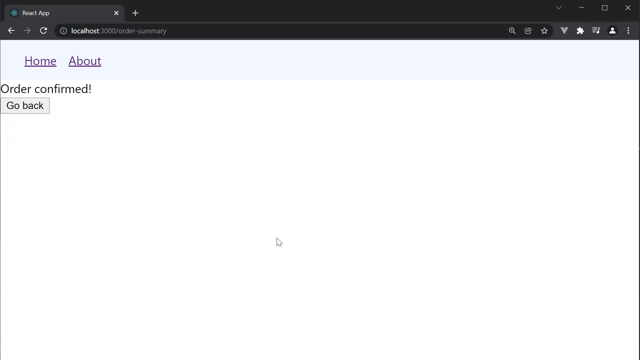 want to go back in the browser And for that we pass in a value of minus one. Head back to the browser and click on go back. We are navigated back to the home page. Place order- go back. Of course, you normally wouldn't go back from the order confirmation page, but I just wanted to show you an example of 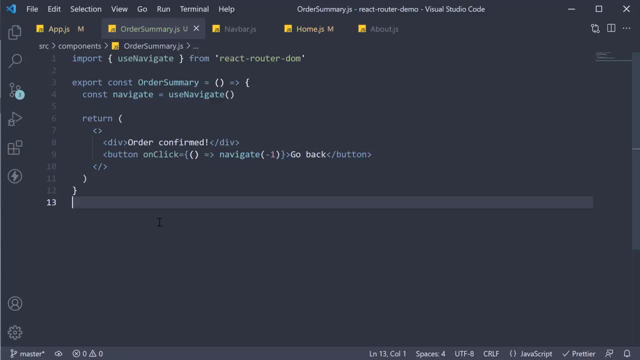 navigating back programmatically. Now you might also want to replace the history instead of pushing a route onto the stack. For that you can pass in an optional second argument. So in homejs to navigate, we pass in an optional second argument. 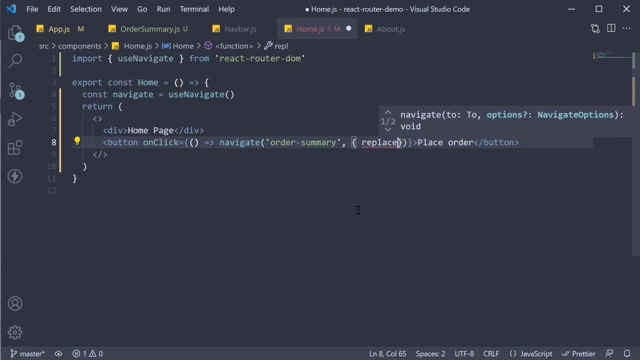 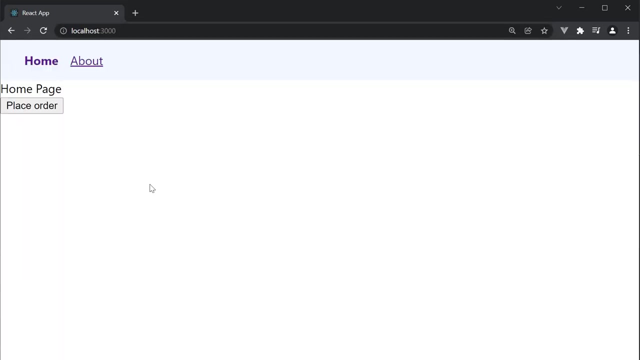 which is an object with a property called replace set to true. Now I'm going to close the browser and reopen it behind the scenes. Local host: port 3000.. Now click on place order. If I now click on the back button, 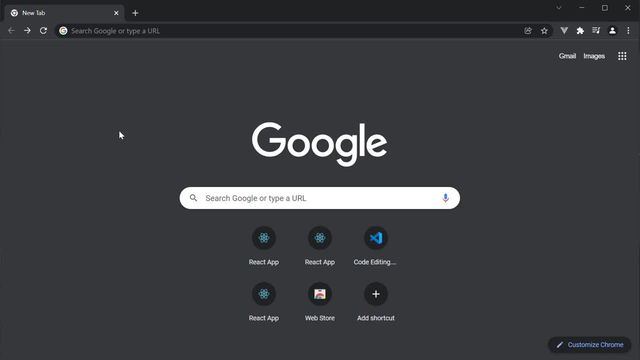 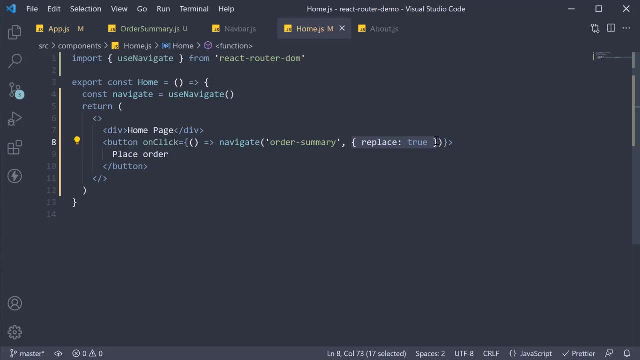 you can see we have come all the way back instead of going back to the homepage. This is because we replaced, instead of pushing order summary onto the history stack. So to summarize, React Router provides the use navigate hook to navigate programmatic Call the hook within the component and use the returned function to navigate, passing in either a path or a number that indicates a change in the history stack.